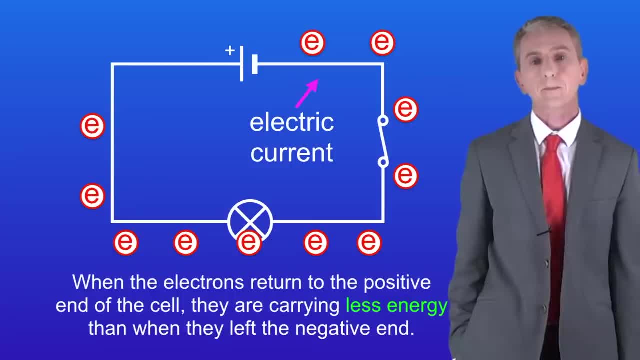 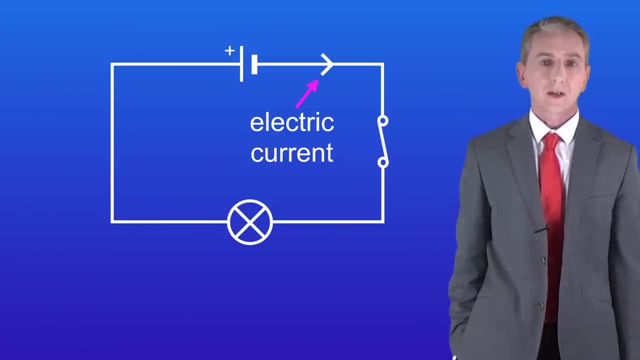 energy is transferred to light energy and thermal energy. When the electrons return to the positive end of the cell, they're carrying less energy than when they left the negative end. We usually represent the electric current using an arrow like this. Now there is one point I need to make here. 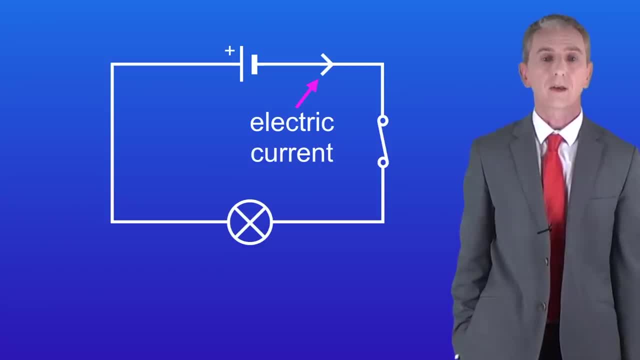 Many years ago, scientists thought that the current flowed from the positive end of the cell to the negative end. We now know that that's incorrect, but we still draw the electric current in that direction. like this. We call this the conventional current, and you're going to see that in all my 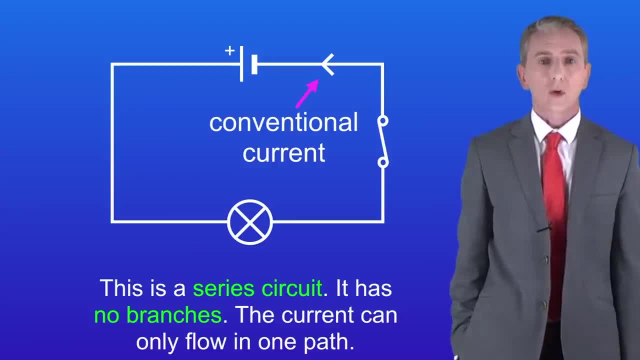 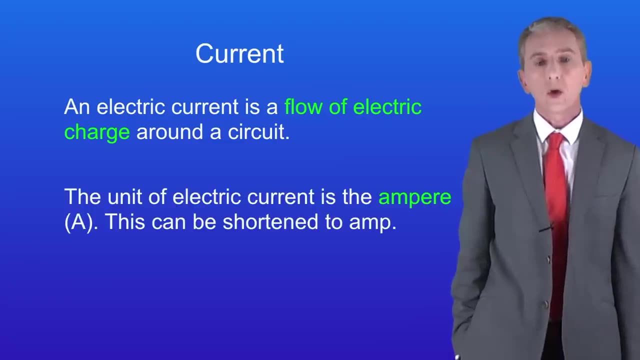 videos. Now, circuits like this one are called series circuits. That's because they've got no branches. The current can only flow in one path around the circuit. So, as we've said, an electric current is a flow of electrical charge around a circuit. The unit of 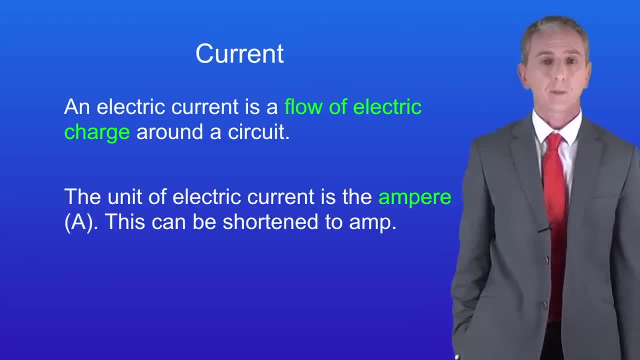 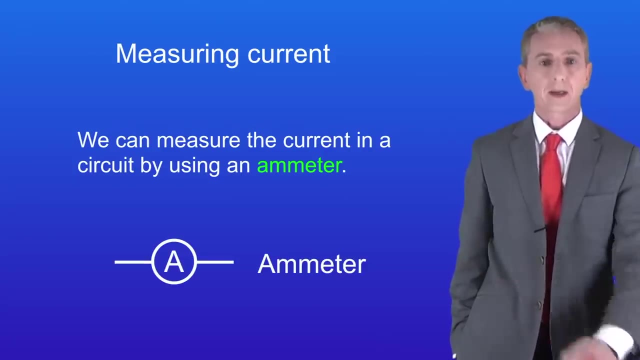 electrical current is called the ampere, and the ampere has a symbol, capital A. Sometimes you'll see the word amp as a short form of ampere, and that's acceptable. Now we can measure the current in a circuit by using an ammeter. Here's the symbol for an ammeter and again, it's really important that. 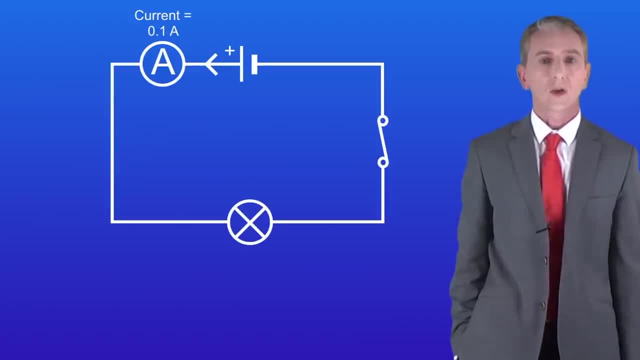 you learn this symbol Okay. so here's the ammeter in our circuit. This ammeter is reading a current of 0.1 amperes. I'm now going to place another ammeter into the circuit, and here it is. This ammeter is also reading a current of 0.1 amperes, and that brings. 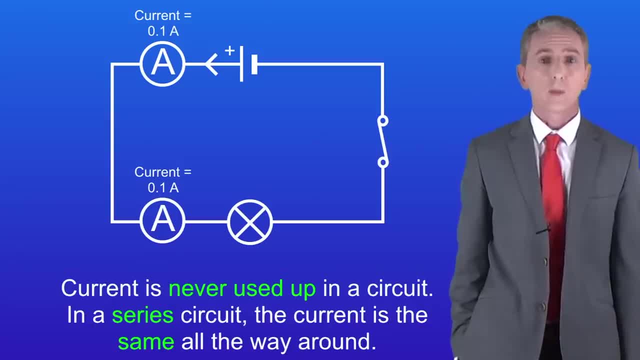 us to a really important point. Current is never used up in a circuit. In a series circuit, the current is the same all the way around. So if I measure the current at this point again, it'll be 0.1 amperes. and here it is. 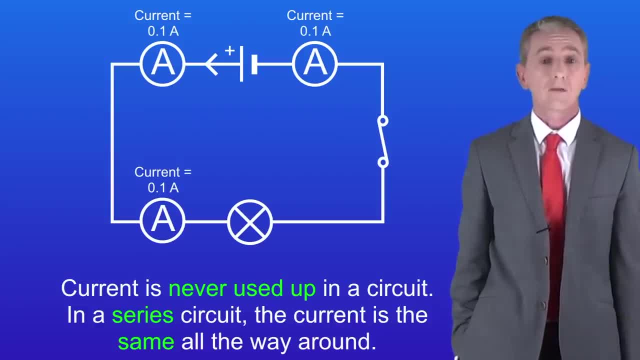 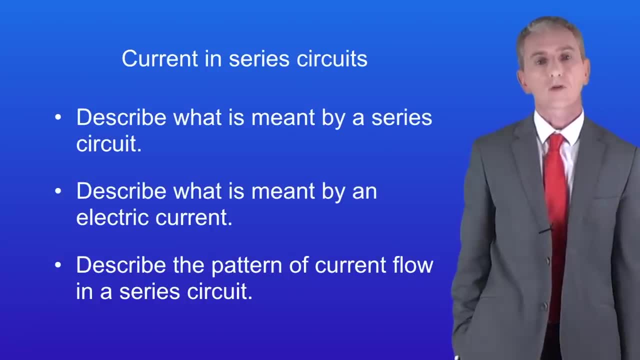 Remember that you'll find plenty of questions on electric current in series circuits in my revision workbook, and you can get that by clicking on the link above. Okay, so hopefully now you should be able to describe what's meant by a series circuit and by an electric current. You should then be: able to describe the pattern of current flow in a series circuit.